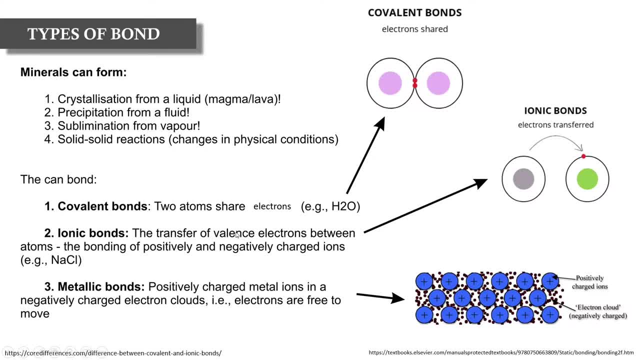 secondly, we have ionic bonds, which is the transfer of valence electrons, so electrons in the outer shell of that element, between the atoms, and this is the bonding of positively charged cations and negatively charged anions, and a good example of this is sodium and chlorine, Chlorine being the. 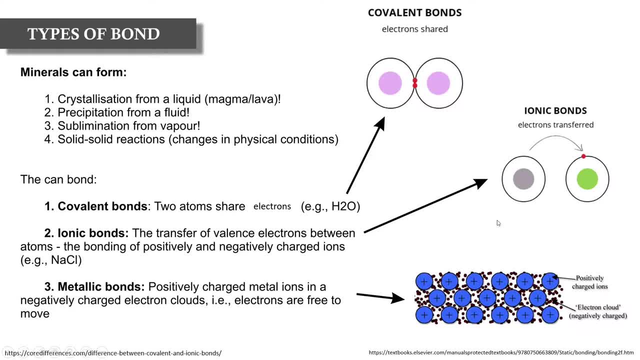 anion and sodium being the cation, and they exchange electrons like this. And then we have metallic bonds, whereby we have a group of positively charged metal ions and metal cations, that's in a negatively charged electron cloud, and this is sort of exemplified in this nice little animation. 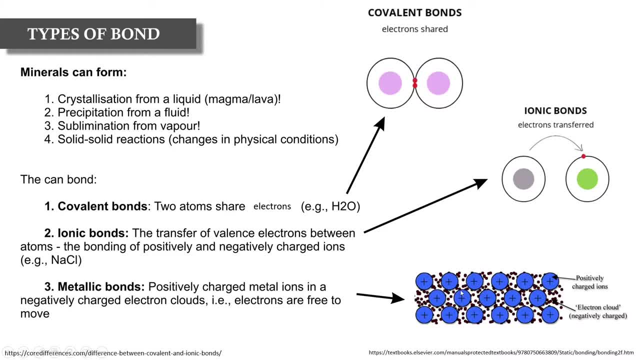 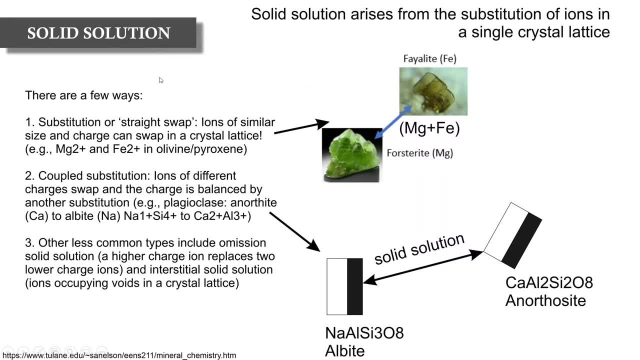 here, where we have electrons that are freely moving around between the metal cations. So solid solution arises from substitution of ions in a single crystal lattice, and there are a few ways we can do this. So firstly, we have substitution or straight swap, so ions of a similar size and 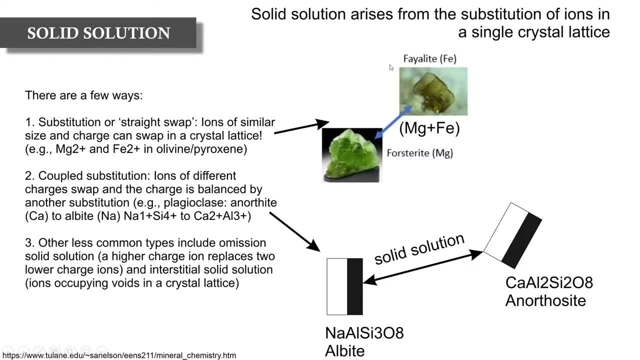 charge can swap for one another in a single crystal lattice. So let's give an example what we have then. so if we give the example of olivine, we have two end members. we have purely magnesium rich olivine, which is known as phosphorite, and then we have purely iron olivine, which is known as phthalite. 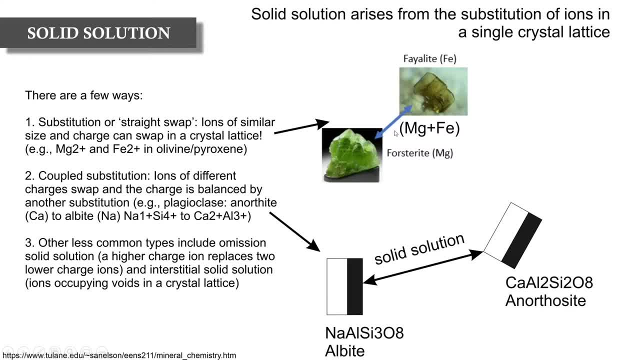 and these two phases form a solid solution in that we can have a mixture of both magnesium and ion in an olivine anywhere in between these two end members. Secondly, we have what's known as coupled substitution, whereby ions of different charges swap and because they have different. 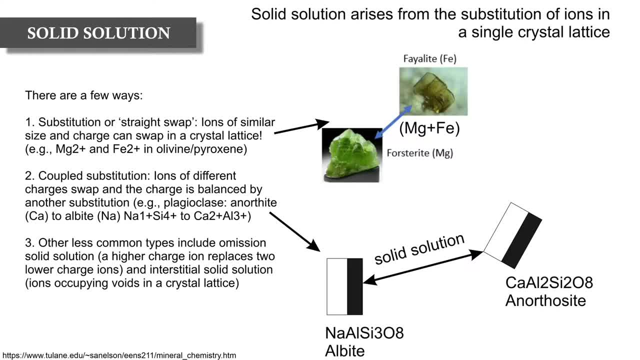 charges, a second swap will need to be made to balance the two end members. So we have a charge in the two phases, and a good example of this is in the plagioclase solid solution series, whereby we have a calcium rich plagioclase known as anorthite, and then we have sodium rich. 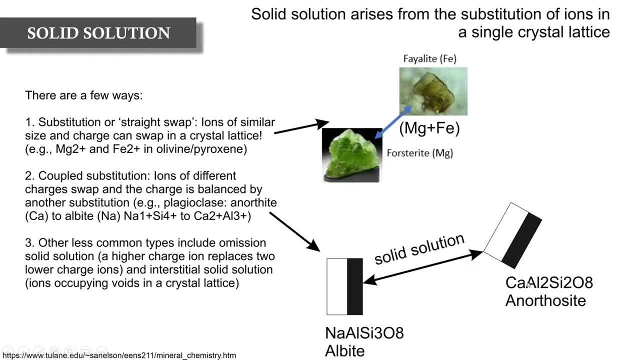 plagioclase known as albite In the anorthite anorthosite being a rock composed of purely anorthite, so apologies for that. so in the anorthite we have calcium as the end member, so it's calcium rich plagioclase. So what we would have to do is we would replace calcium 2 plus by 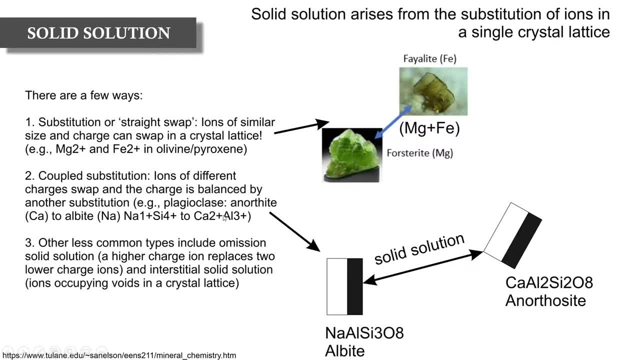 because you know sodium is 1 plus and calcium is 2 plus, we have to complete a second substitution. so we would replace an aluminium 3 plus with a silicon 4 plus element to balance the charge, and that's why we have two aluminium ions here and two silicon ions here, whereas in albite we 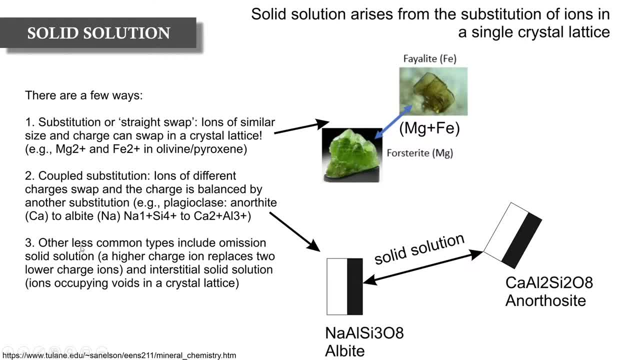 have one aluminium ion and three silicon ions. And thirdly, we have some other different types of solid solution whereby we have what's known as emission solid solution, whereby a higher charge is applied to the ion in the solution, and then we have the interstitial solid solution, whereby 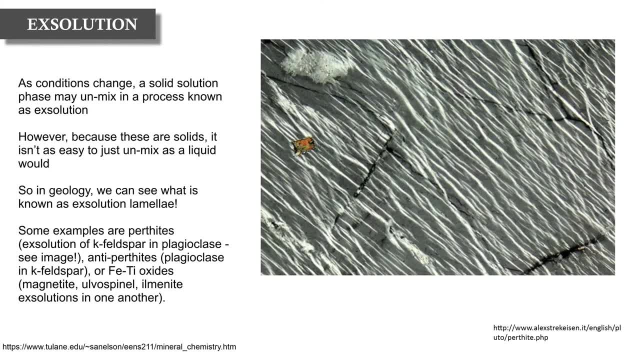 ions occupy voids or spaces in crystal lattices. So exsolution is a process whereby a phase that is initially in solid solution will become unstable due to changes in conditions and it will try to separate into two different solid phases. but because these are solids and not liquids, the 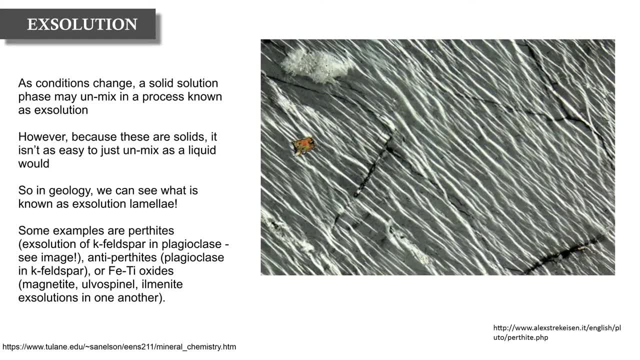 process of separation is quite difficult. so instead of forming two individual phases, we form what's known as exsolution lamellae. so we have exsolution lamellae of one phase that's been formed and a larger phase, and a common example of this is in granites. so in granites we have 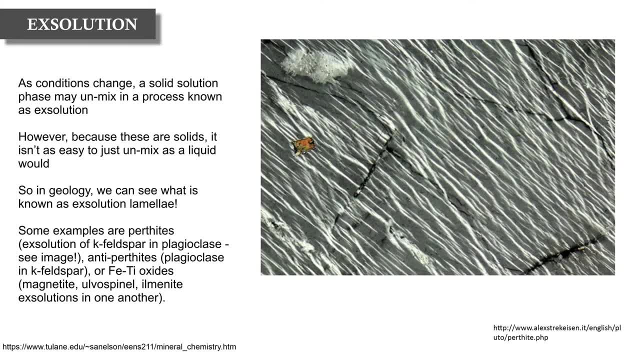 typically alkali or plagioclase feldspar phenocrysts. so we have quite large feldspars. so if we take a large alkali feldspar, we can exhibit what's known as perthite or perthitic texture. and what that is is: we have our alkali feldspar and within it we have exsolution lamellae of 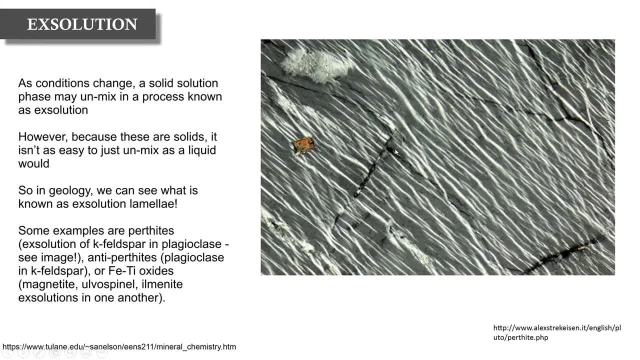 plagioclase, and this is essentially all the calcium and sodium escaping from that crystal lattice of alkali feldspar because it is no longer compatible with the solid solution. so this is what we're seeing in this photo micrograph. here we have exsolution lamellae of plagioclase within a large alkali feldspar. the opposite of this would be: 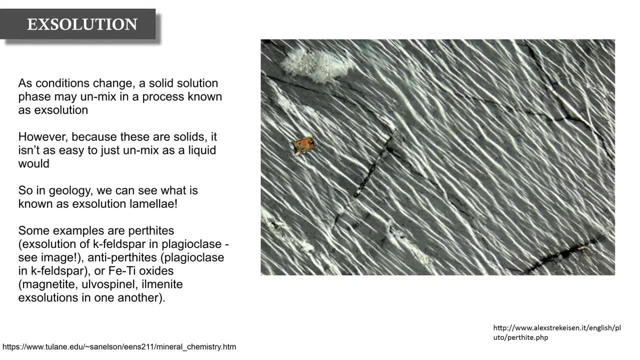 antiperthites, which is we have plagioclase phenocrysts and then exsolution lamellae of k-feldspar. there are some other examples of this in geology, iron oxides being another common one, where we have things like magnetite, titanomagnetite or ilmenite exsolutions in one another, and 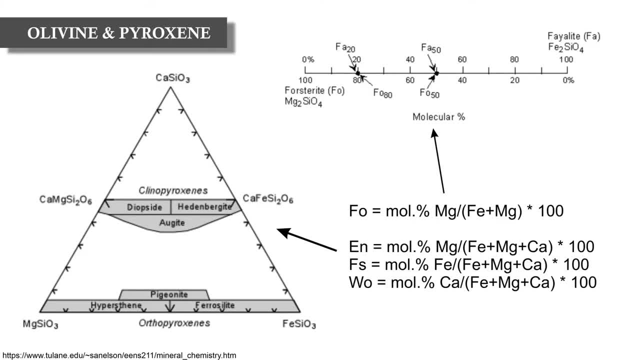 there's obviously several other examples as well, so we can calculate the composition of phases through some fairly simple calculations. so first, if we take a look at olivine up here, we can calculate what's known as the forstright or phthalite number, forstright being fo phthalite. 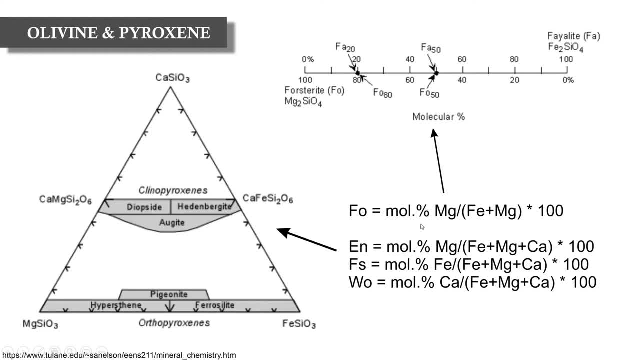 being fa, and essentially the calculation for magnesium number, where we calculate molar magnesium divided by molar iron plus magnesium multiplied by 100, and then we can generate olivines anywhere on this spectrum. here, where we have two n members, we have 100 iron here, as you. 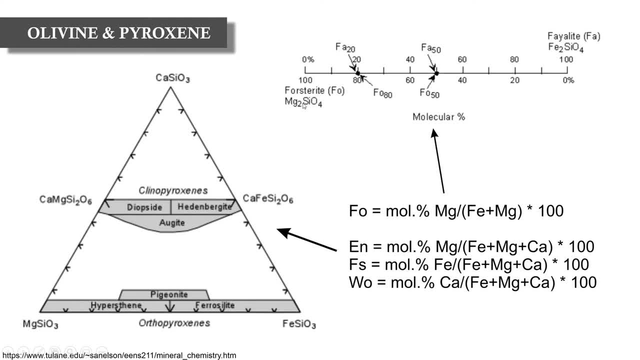 can see by that formula in what's known as phthalite, and then we can calculate the forstright and then we can have a spectrum of different olivine compositions in between and we typically, when a magma crystallizes and it is olivine saturated, it will precipitate. 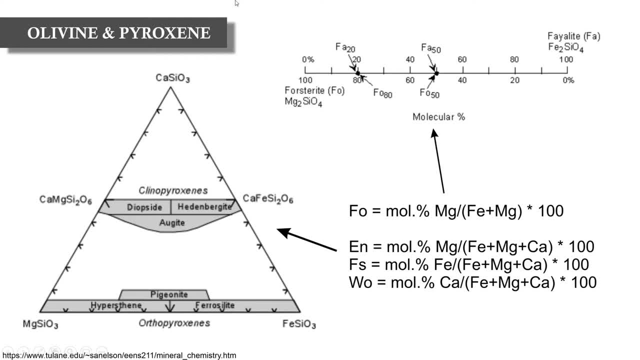 the most magnesium rich olivine, and typically the most magnesium rich olivines that can be produced in nature, is around 93 percent forstright. so what we can see here. so if we had a spot here, which we do in this example, we have 80 percent forstright or 20 percent phthalite, and then we 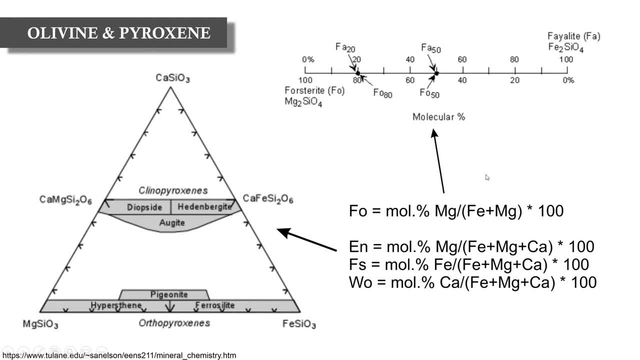 calculate that forstright, so this would typically be denoted as fo 80, and that's the result of this calculation. here, if we take pyroxenes, we're adding a third n member. so not only do we have the solid solution series here between magnesium and iron, we've thrown calcium into the mix, so we have 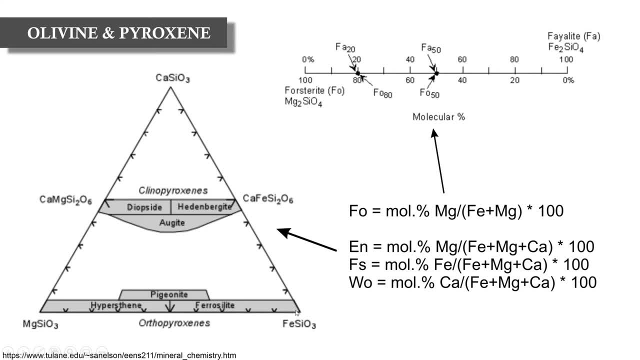 enstatite down here, we have wollastonite up here and we have ferrosylate down here, and then we have another solid solution in the middle for our clonopyroxenes. so the calculation operates exactly the same as forstright, except we've also added in calcium, and then we would analyze our 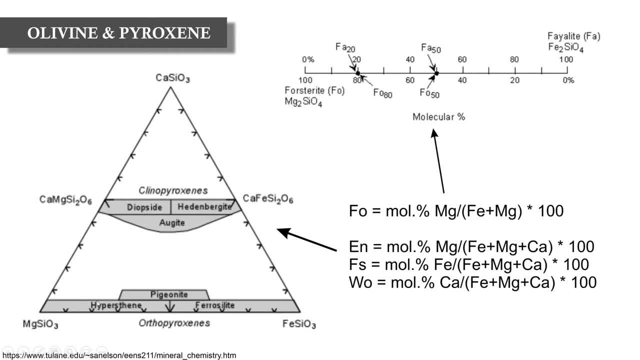 minerals, and they would plot somewhere within this ternary diagram and then we would be able to determine the type of pyroxene that we've analyzed here. we have sort of gaps whereby there's no natural occurring phases in nature, and that brings us on to feldspar's, so similar to pyroxenes we 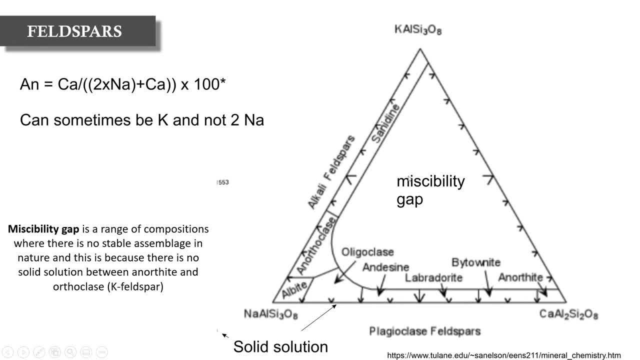 display it as a ternary diagram. but, as you see, they're slightly different, as in we have what's known as the miscibility gap. so, firstly, we have anorphite down here, which is our calcium rich end member, we have albite down here, which is our sodium rich end member, and we have